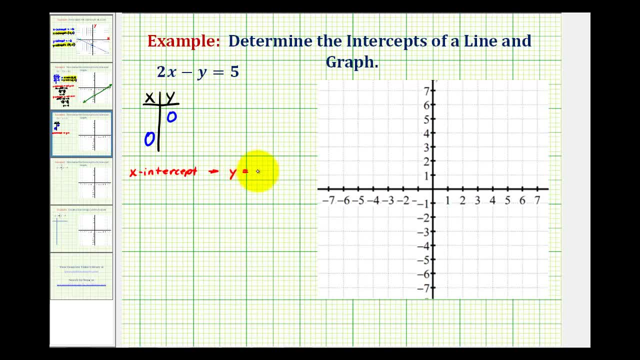 Let's go ahead and do that below. Let's start by determining the x-intercept. So again, we're going to let y equal to zero and solve for x. So if we let y equal to zero, notice how this term here would be zero. 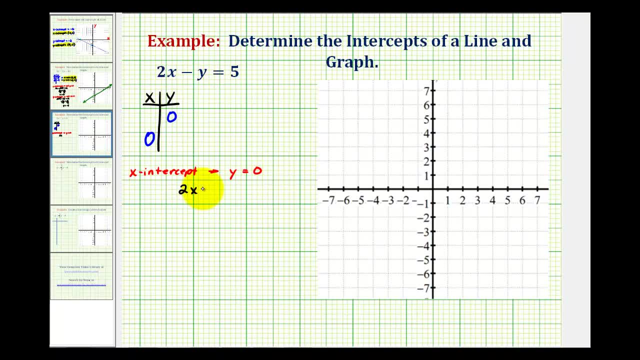 So we'd be left with 2x equals 5. And we divide both sides by 2. We have x equals 5 halves, which would be our x-intercept. So again, the x-intercept, It is the point 5 halves zero. 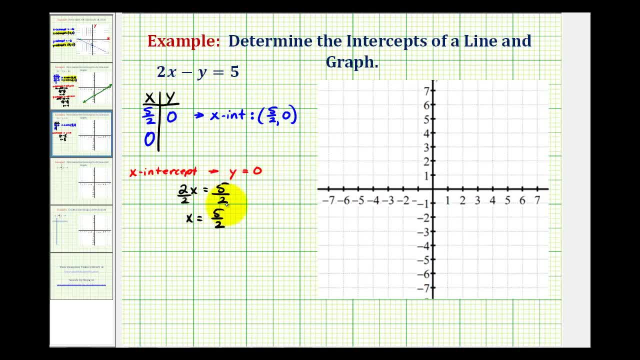 And it might also be helpful to write this as a mixed number or a decimal: Five halves, or 5 divided by 2 would be equal to 2.5.. Now we'll go ahead and determine the y-intercept And, as I said before, we're going to set x equal to zero and solve for y. 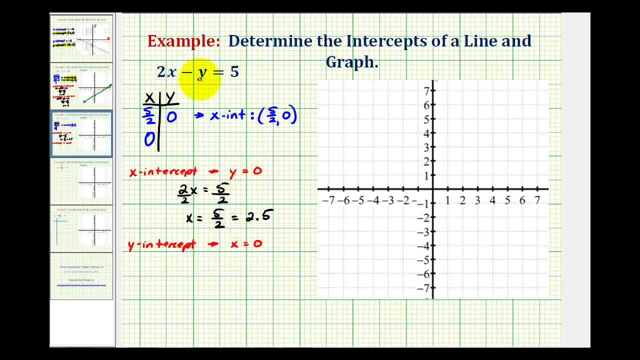 Notice: if we set x equal to zero, 2x would be zero, So we'd be left with 2x. And if we set x equal to zero, 2x would be zero. And if we set x equal to zero, 2x would be zero. 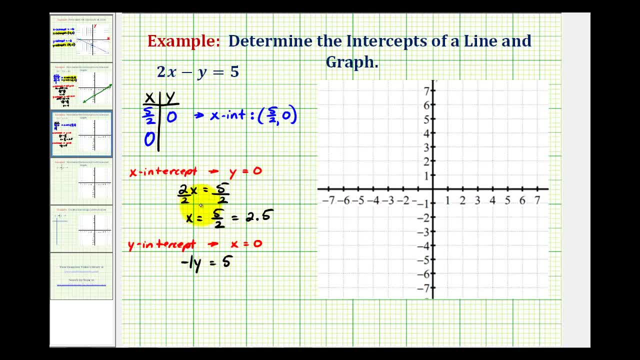 And, if it's helpful, we can write this as negative: 1y equals 5.. So to solve for y, we'll divide by negative 1. So we have y equals negative 5. So when x is equal to zero, y is equal to negative 5.. 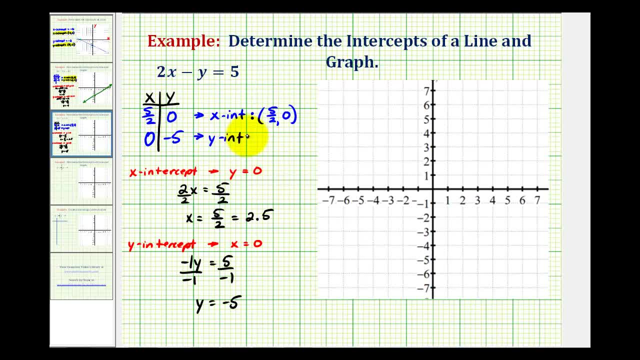 Therefore the y-intercept is the point zero negative 5.. Now it is important that we don't forget that We don't list the x-intercept as just: x equals 5, halves or 2.5, because technically that's the equation of a vertical line. 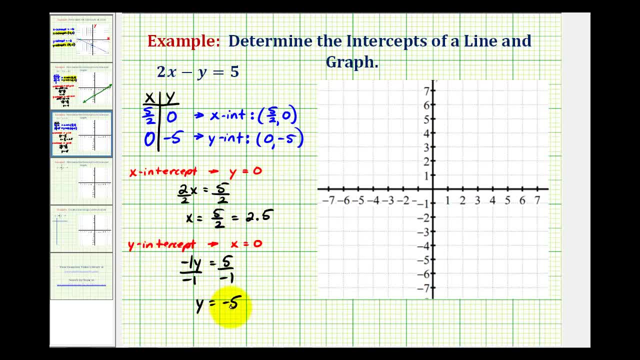 And we also shouldn't list the y-intercept as just y equals negative 5, because that's an equation of a horizontal line. So we should either give the intercepts as ordered pairs or state the x-intercept equals 5 halves and the y-intercept equals negative 5.. 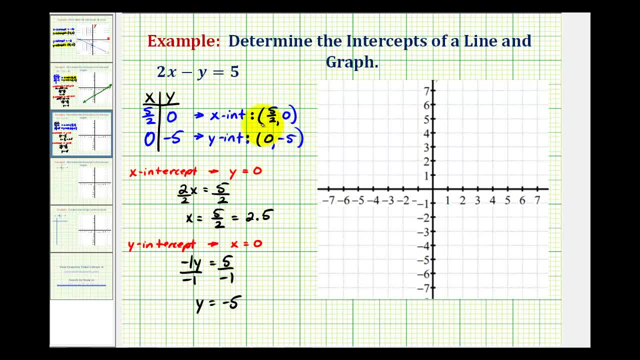 Now let's go ahead and plot the intercepts and then sketch the line. So the x-intercept is 5, halves zero, Or 2.50, so the x-intercept would be here, And then the y-intercept is the point zero negative 5, or this point here.